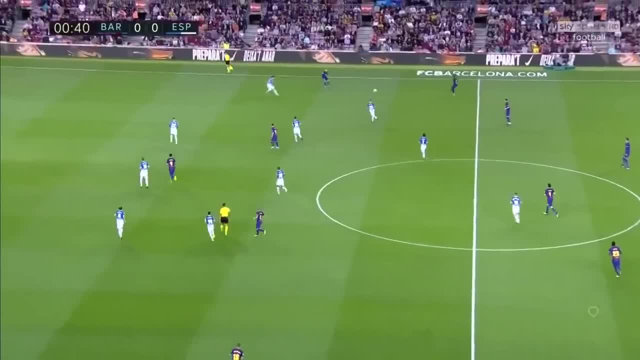 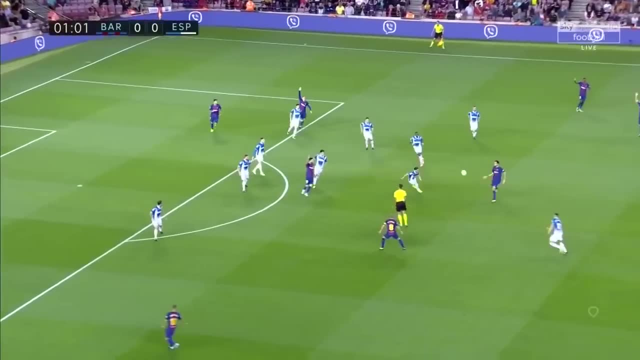 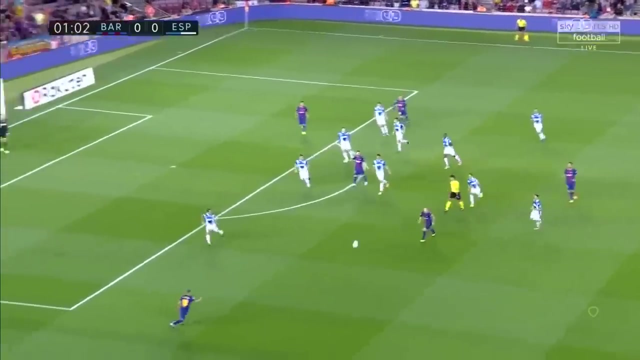 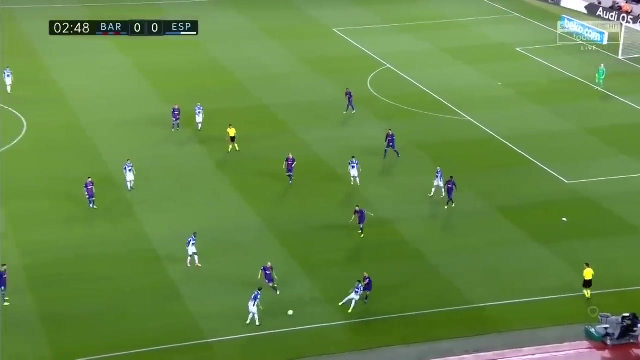 As a center back, almost just in case for that counterattack. He's coming back in the center and he's really just kind of staying in the center available. And now he's going to get the ball bounced up to him and immediately watch how busy it is and how many people are over on that right side of the field. So without hesitation he one touches it over to his left mid, Then on this play, watch he's guarding here, He's guarding here. And then you'll see the moment he looks over his shoulder, realizes this guy is too far back, pass him onto a center back almost instantly just to occupy that space. Just a little bit of help defense. 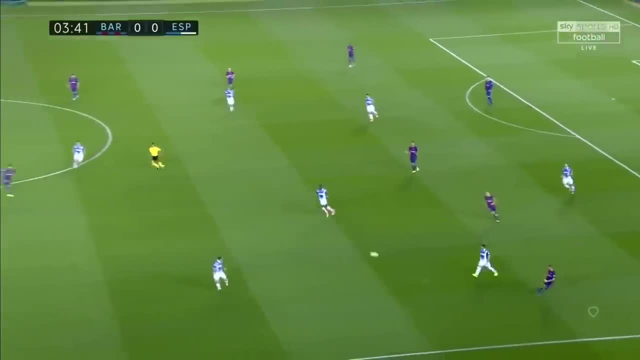 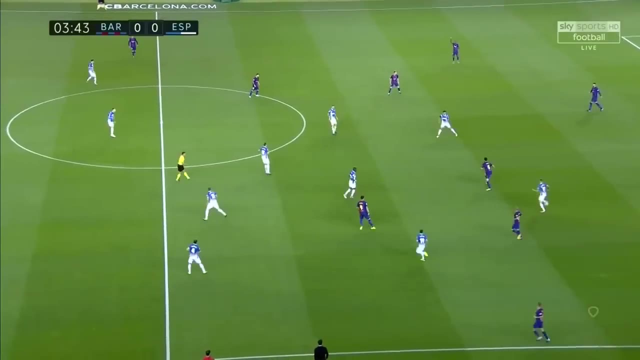 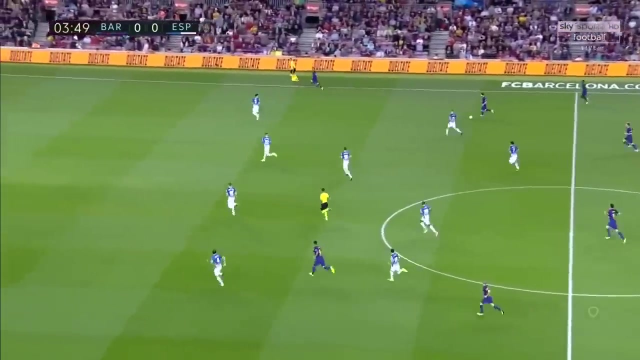 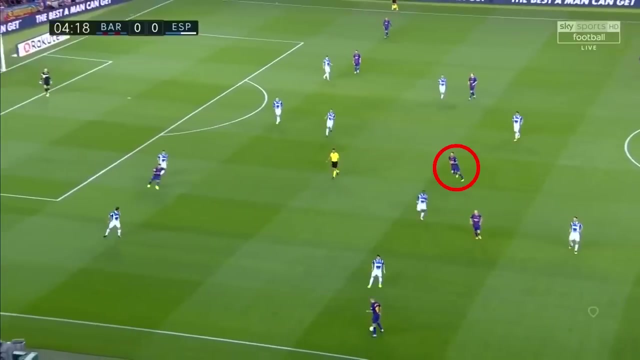 Now this is something that you'll see. center mids do a lot. Watch as this ball goes into the forward. watch Busquets almost come underneath him in a pocket of space to receive that drop pass from that holding forward And now he has the ball facing the field and can switch the point of attack and look forward. Now same exact thing from Busquets, again, Watch it's going to go out wide and it's going to go into the forward and he's already moving to get in that pocket of space beneath him, Receives the ball and now can turn and attack and face the field. 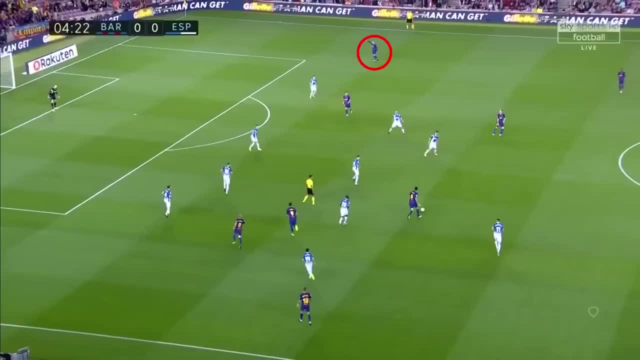 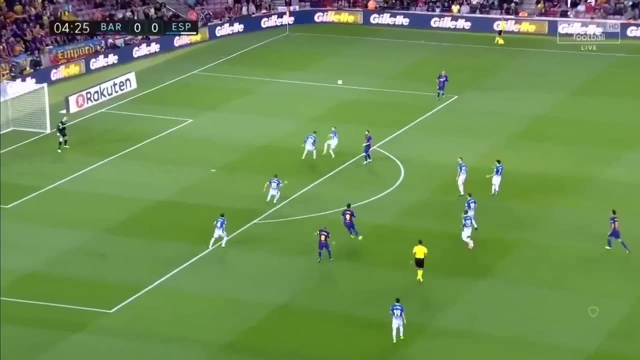 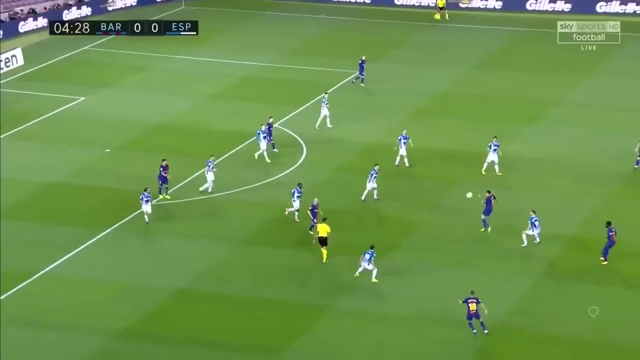 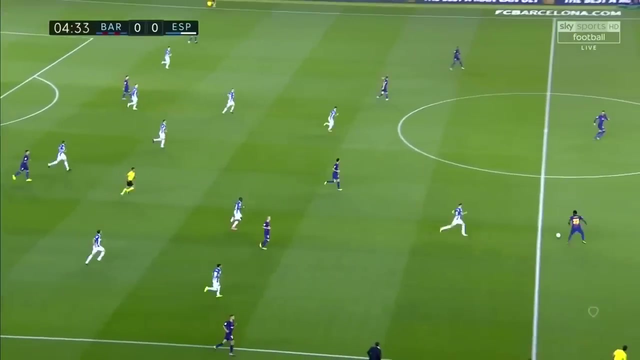 And now I thought he was going to hit a long ball all the way over here, but he instead does something that only Busquets, I think, can do and plays it into Messi here and threads the needle. Now watch as this ball is bouncing around. It's cleared out right here. Busquets checks his shoulder really quickly. He already knows that defender is on his back so he can head it out wide and not bring it down, trap it and then probably get tackled. Now, if you were to take away one thing from Busquets' game, I think it's this, and it's this ability that he always finds like a pocket of space, And what 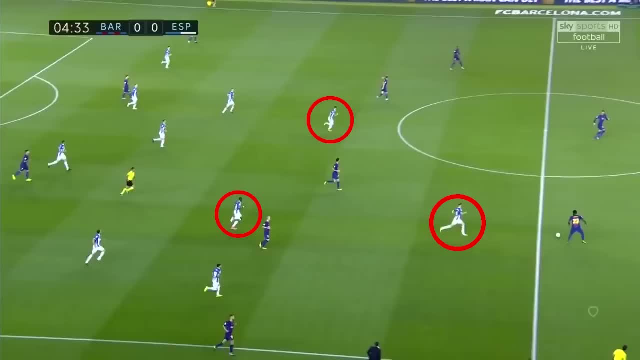 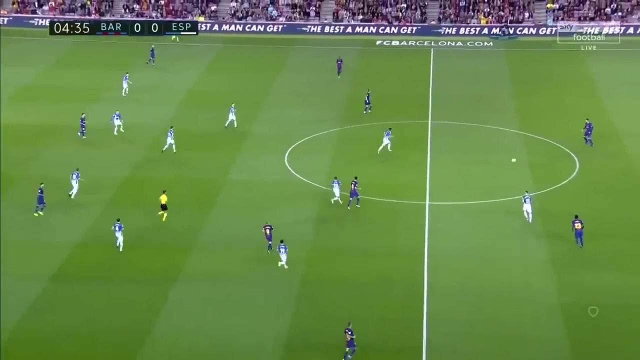 I want you to watch. So right here, this is between one, two, three defenders. This is like in the center, epicenter of a triangle, And you'll see this happen again and again, and again. and just watch and learn, if you're playing center mid, about how good at this Busquets is. So let's go into this play and watch how much time and space he gets because of his positioning. So he gets the ball and as the ball is played now, he has tons of time to be able to receive it. and then one touch to the other defender And watch, even now, in the center of the. 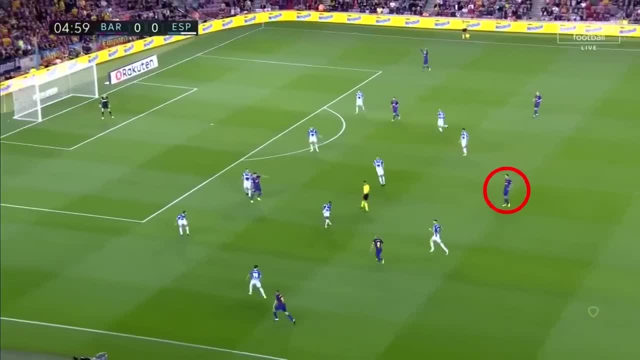 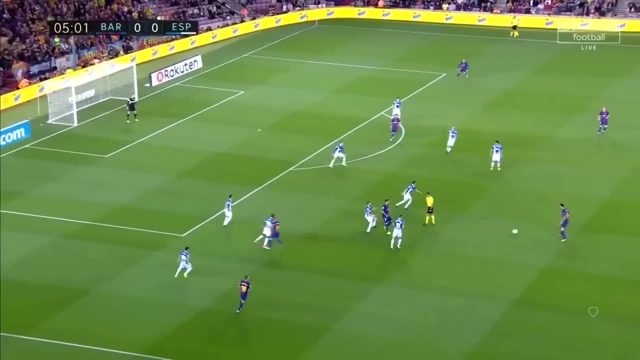 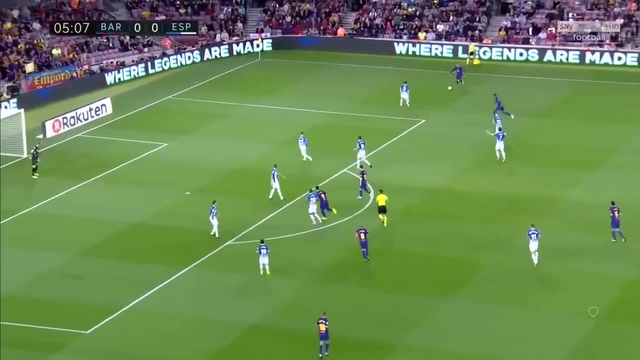 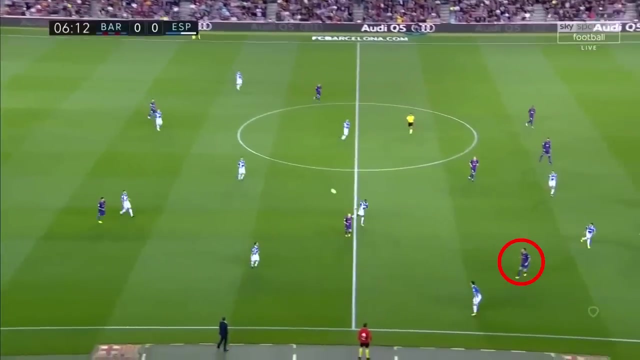 triangle. Now watch Busquets predict this. So he's walking to the left and right. here he stops because he knows this ball is about to be played in and everybody's moving to the left. So he has lots of time and space so he can receive the ball, turn and now play to the other side. It's just little things like that how he creates space for himself. He's doing opposite of what everybody else is doing and moving into those pockets of space constantly. Okay, I just want you to watch Busquets' movement right here and notice this very small thing. So watch as that ball comes into this guy. 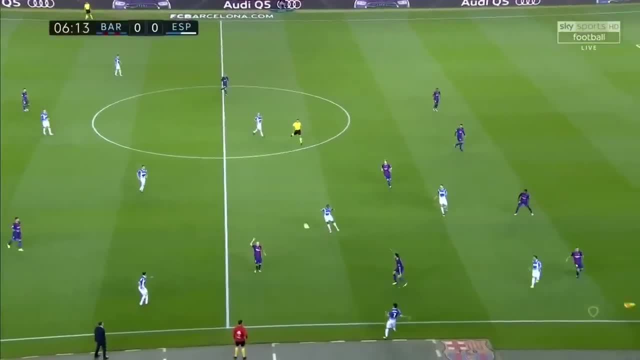 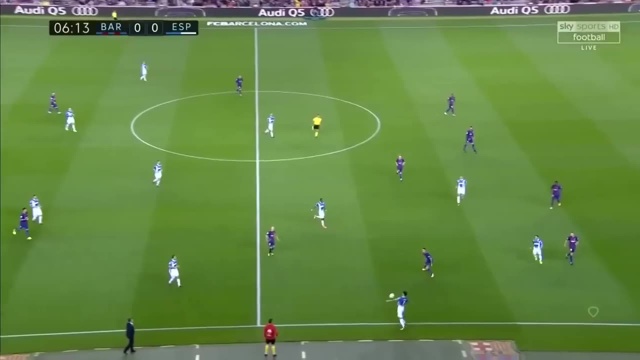 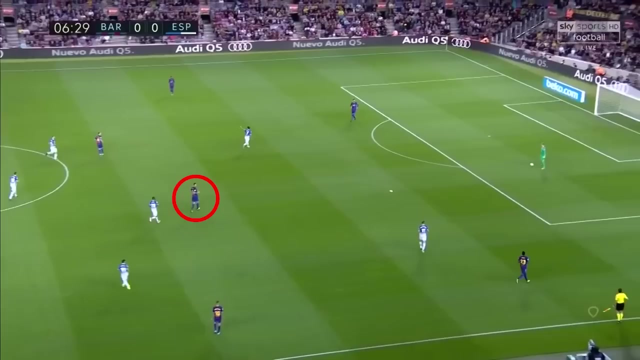 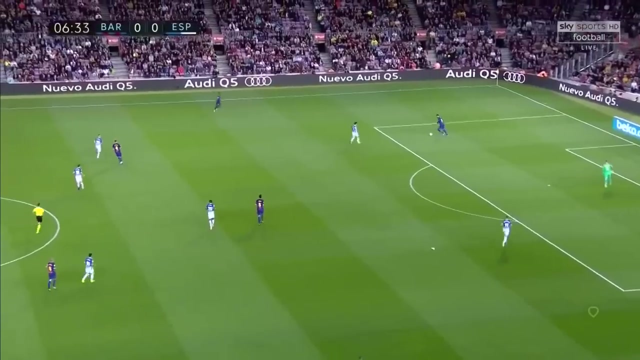 Instead of Busquets running at him very fast and just trying to defend him, he backs up to almost predict like he's going to hit that first time to this guy right here to intercept that pass. Very, very cool and just a very veteran play. Now in this play I just want you to notice Busquets' movement in general He's always creating a passing lane- him and the goalie right there As the ball goes out to that right center back. now there's a passing lane between him and that right center back As it goes in that right back now there's a passing lane between him and that right back As it 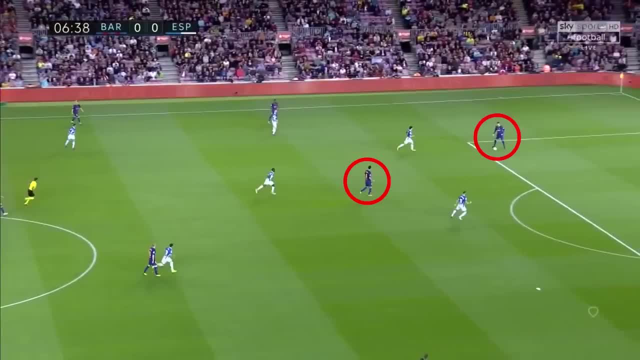 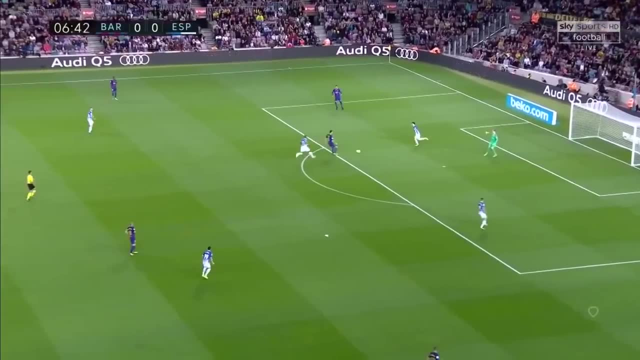 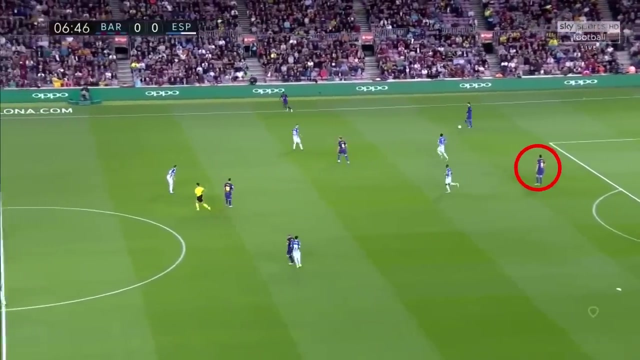 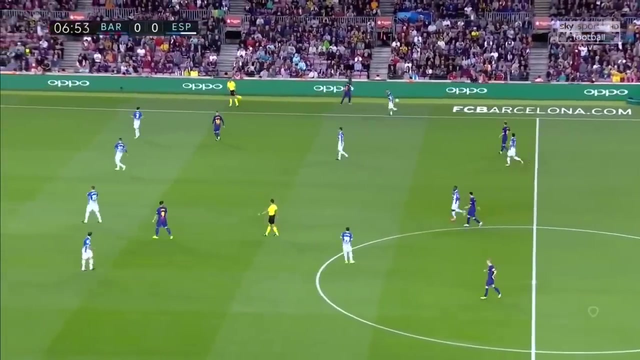 cuts back and plays the center back. there's a passing lane between him and that center back. Again, now it goes to the goalie and he's checking to create a better passing opportunity for that goalie to pass to him and immediately notices pressure, plays it out to the center back. He's always moving to create these passing lanes. Even watch right here he stops to create a passing lane for that outside center back, Constantly in a position to receive the ball and create opportunities for his team. Now here he doesn't even get the ball. but again, same concept as before: Watch his movement to. 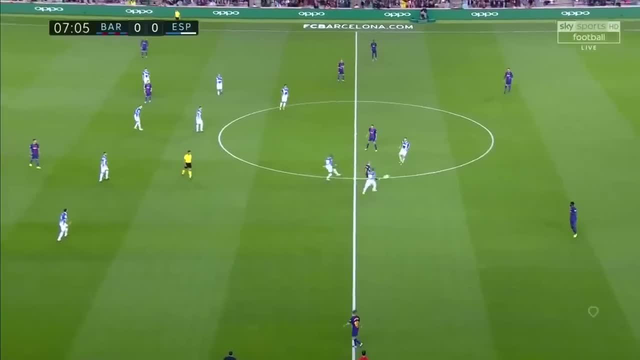 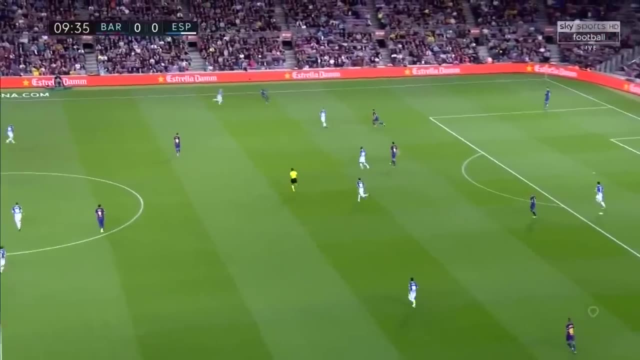 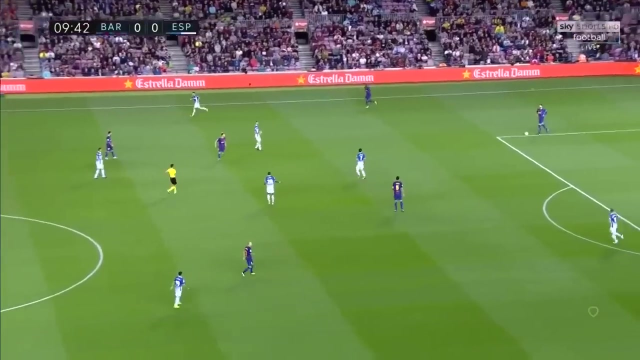 create a passing lane. As it gets closed down here he's shifting to his right to keep that passing lane between him and Iniesta. I think Just constantly. great off-ball movement from Busquets, something that all defensive center mids can learn from definitely. Now here becomes. 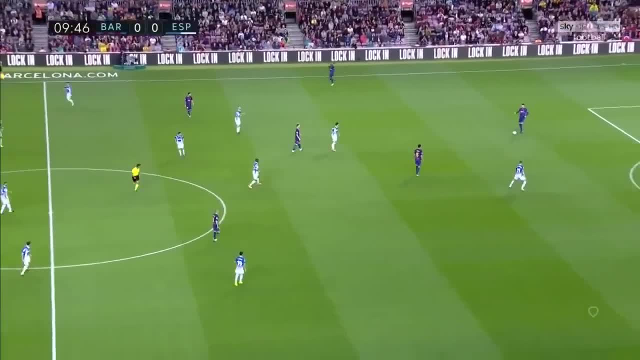 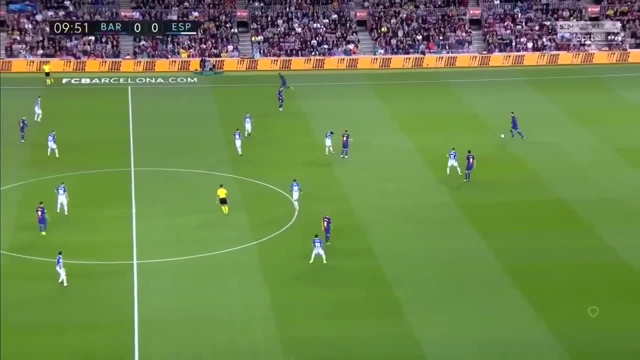 the triangle thing that you'll always see, always in the center of the triangle, always so that he can get the ball and have more time and space to turn and decide what he wants to do with the ball. There's not a guy breathing down his neck because he's always finding that pocket of space. 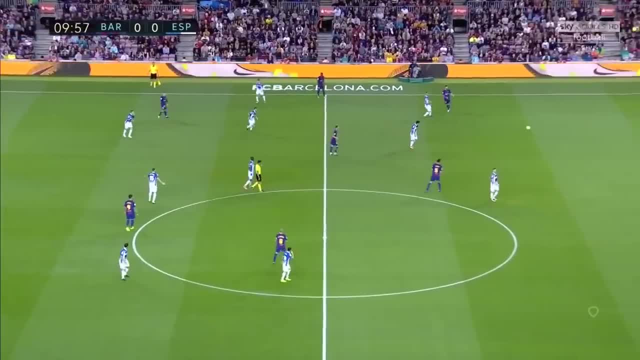 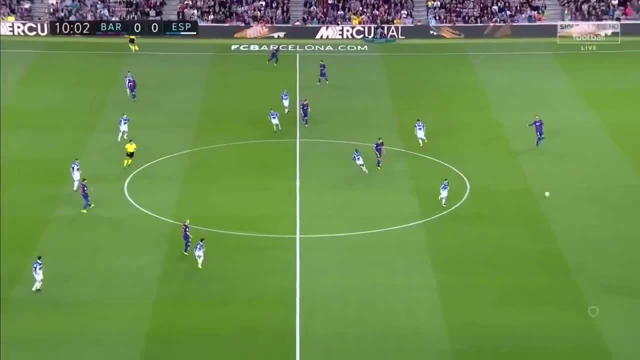 all the time. It's amazing and I mean it's very hard and I mean it's very easy to take that for granted, because even look right now in the center of that triangle so he can receive the ball with a little bit more time and space In that center of the triangle, he's just always moving checking. 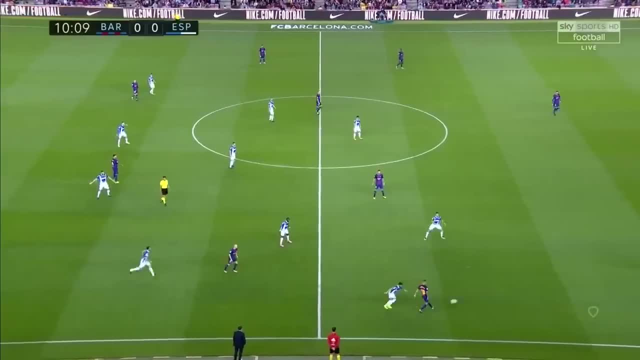 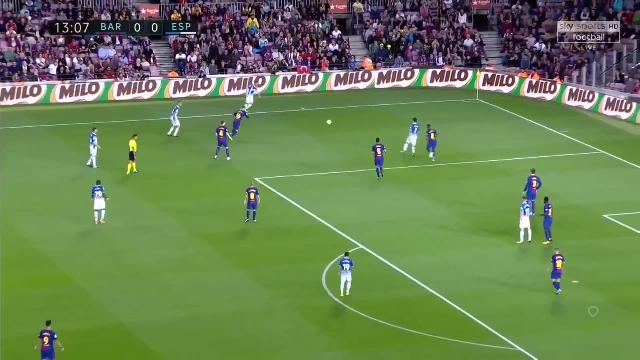 his shoulder, positioning himself. So if he were to receive that ball, he'd have enough time to pick his head up and find where he needs to go next. Very cool and something that everybody can learn from. Okay, now watch. he's just kind of helping defense right now and watch as he shifts to his 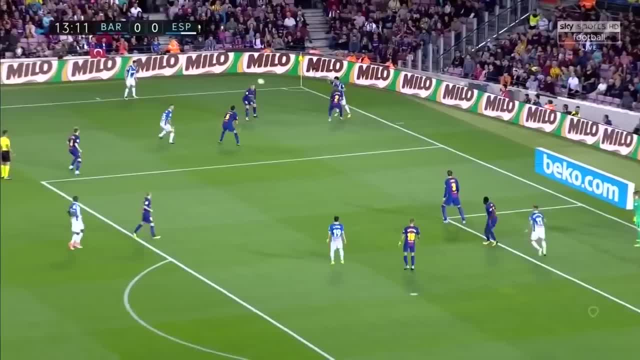 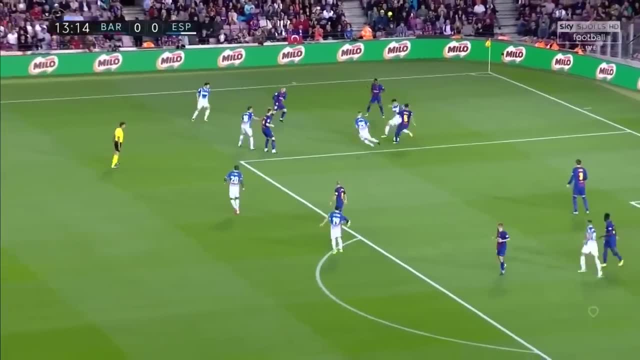 left, right there to block that pass to this guy right here And as soon as that ball goes over his head, watch as he backs up, as it goes into Rakitic to create a little bit of space. so now he can receive the ball and play out of it and he shows some class there with that pull back drag. 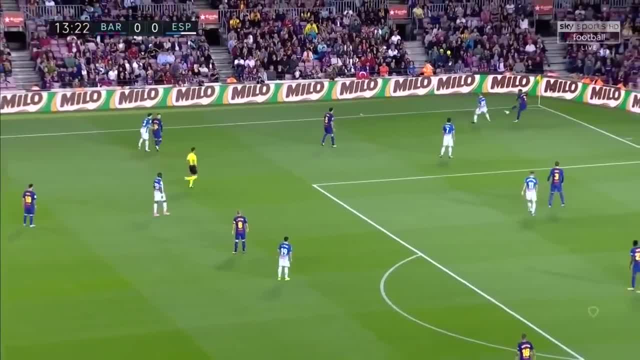 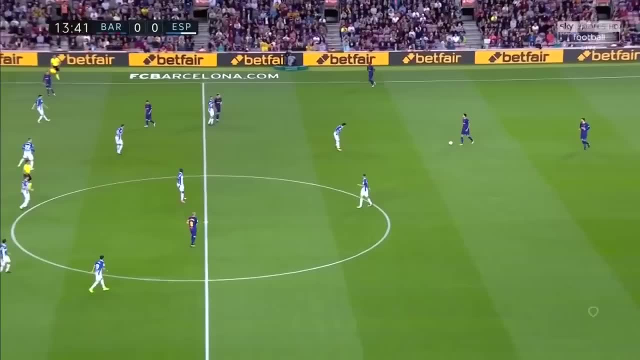 move, But nonetheless his off-ball movement is just world-class and that's why he's a world-class soccer player, given those technical skills as well. Anyway, he gets the ball, he's got the ball here, he turns, he has lots of time and space, he picks his head up, But, as you can see, 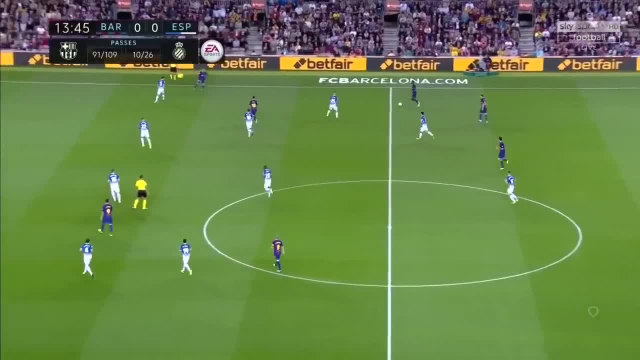 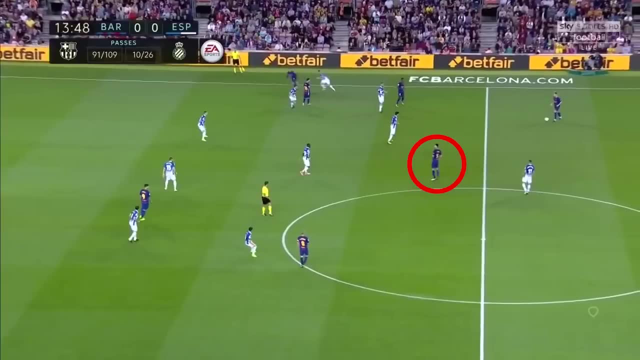 there's no clear-cut option. I at least think. Plays out to his right back, plays a simple pass, just so the team can get the ball moving And then watch this. this is kind of cool thing from Busquets. Busquets looks over his shoulder right here and then he basically tells his center back. 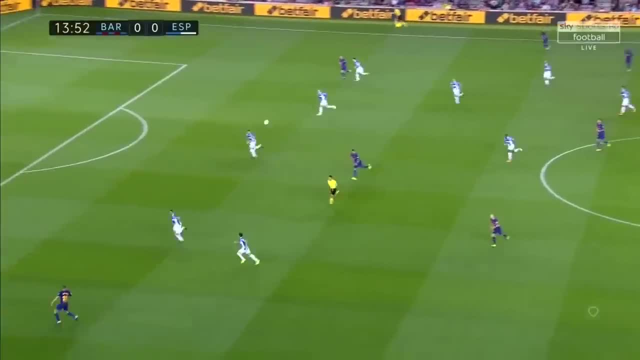 hit that long ball over me. Just a little communication. you can see his like soccer IQ right here, kind of cool On this play. I just kind of want you to notice just him kind of predicting where that open space is going to be, So you're going to be able to see where that. 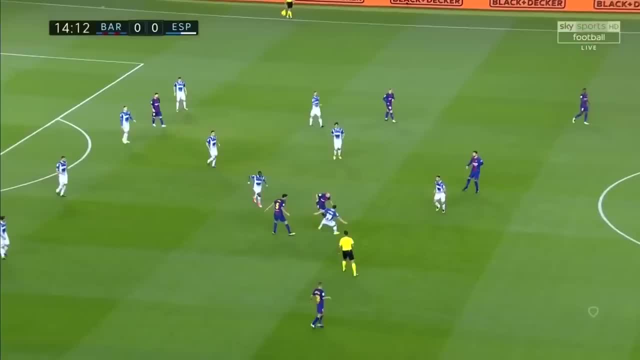 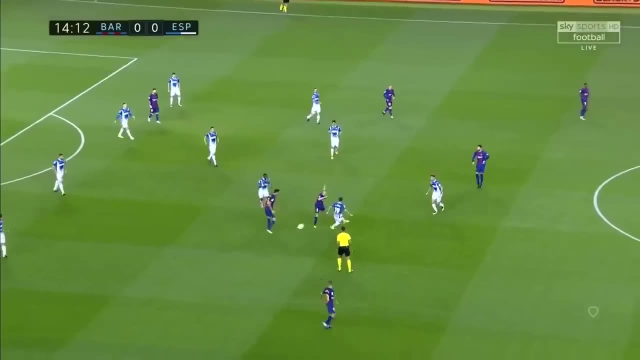 open space is going to be. So you can see him already turning as that ball's played to him. He's recognizing that Iniesta is probably going to play to him. He's recognizing there's a guy to his left and to his right and the space is behind him And he just executes that very simply. 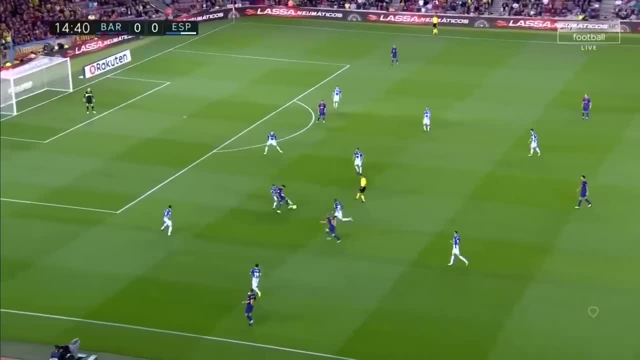 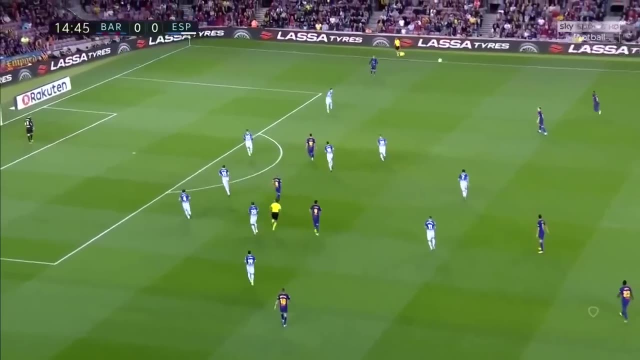 but very professionally. Okay, on this play, just watch. So as that ball goes into the forward, he's splitting between these two defenders, gets the ball immediately, recognizes it's too tight and does an amazing pinpoint- switch over to the other side of the field- Again, world-class. 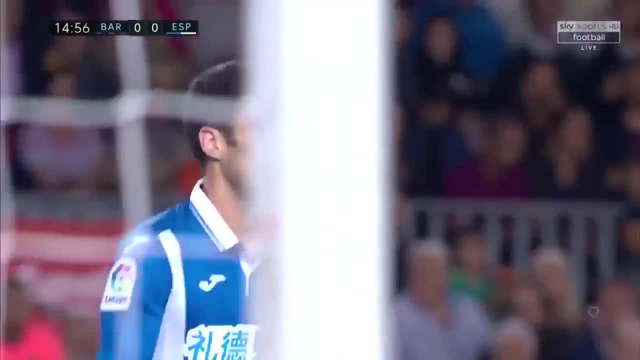 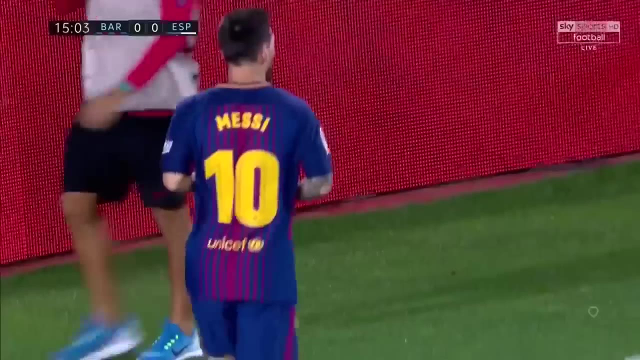 this is why he's at Barcelona, playing where he's at. So anyway, that's pretty much the video. I just wanted to analyze 15 minutes of this game just because I could go so in-depth. and if I analyzed the entire game it'd be a two-hour long video. So I hope you guys enjoyed it. I hope you.